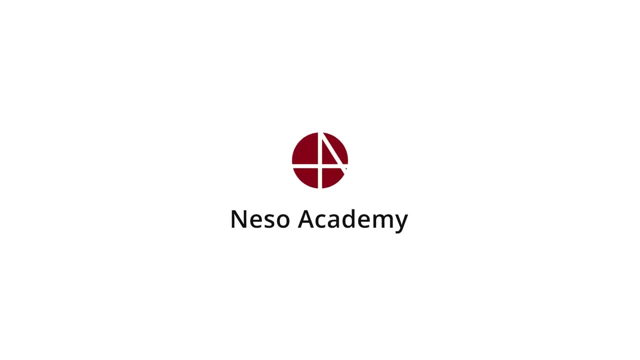 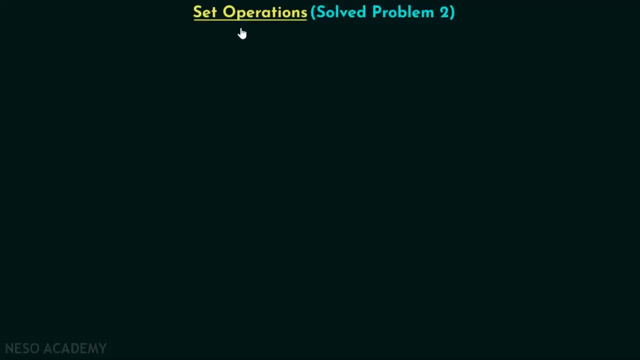 In this presentation we will try to solve problem 2 on set operations. So let's get started. Here is the problem. Draw Venn diagrams for each of these combinations of the sets A, B and C. So we have all these combinations. 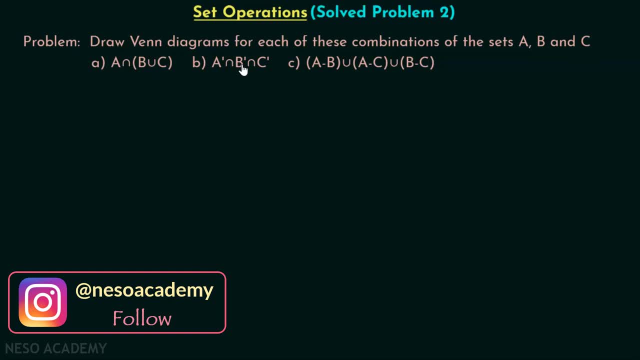 A intersection B, union C. A complement intersection B complement intersection C. complement A minus B. union A minus C, union B minus C. We have to draw Venn diagrams for all these combinations. Let's consider option A, ie A, intersection B, union C first. 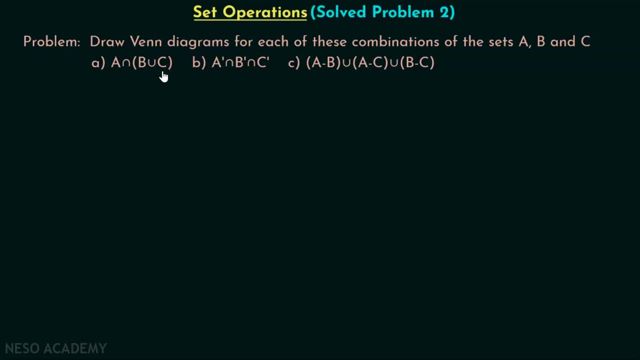 and try to draw the Venn diagram for the same. First we will see how a Venn diagram for A, B and C looks like. This is how it looks like. Obviously we must have a rectangle which represents universe of discourse or universal set. 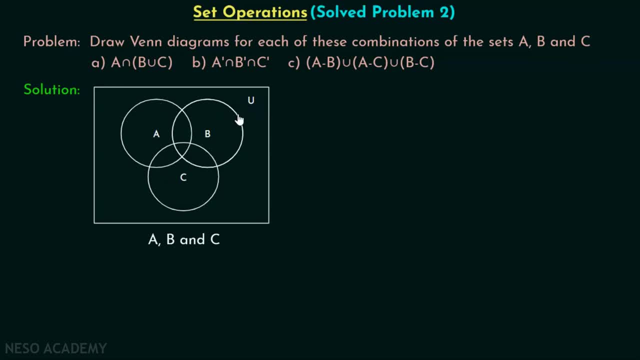 And we must have three circles overlapping inside this region. As you can see, these are three circles And here this circle represents set A, This circle represents set B And this circle represents set C. So this is the Venn diagram for A, B and C. 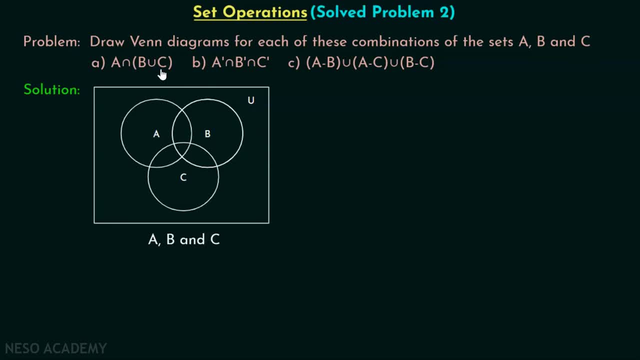 Now we want to draw the Venn diagram for A intersection B union C. First we will try to draw the Venn diagram for B union C, Then we will draw Venn diagram for A intersection B union C. Okay, B union C means everything of B and C must be included. 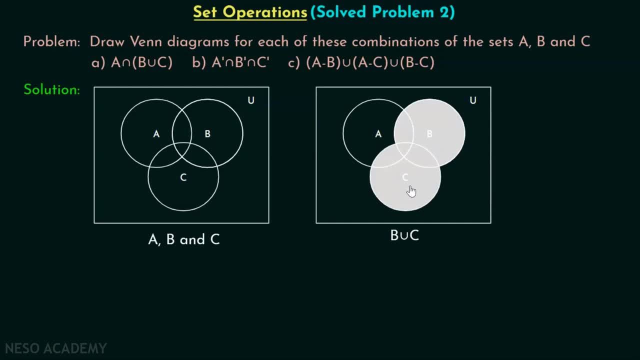 In other words, we can say that either B or C or both Right. This area is common between B and C. This must be included. This area is only B and this area is only C. These two must also be included. So this is the Venn diagram of B union C. 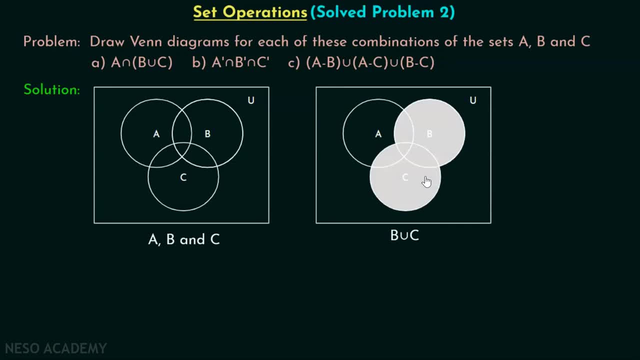 The shaded region represents B union C. Okay, Now we can easily draw the Venn diagram for A intersection B union C. We want the common area between A and B union C. Right. As you can see, this area is common between A. 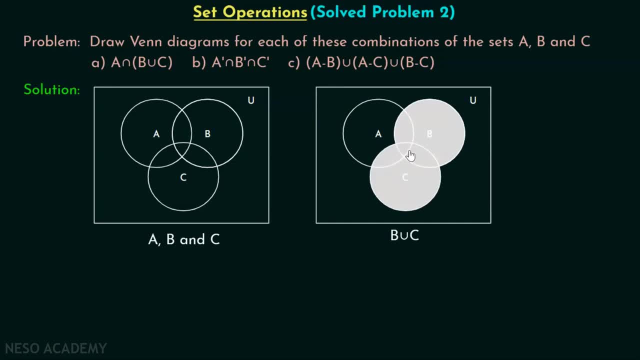 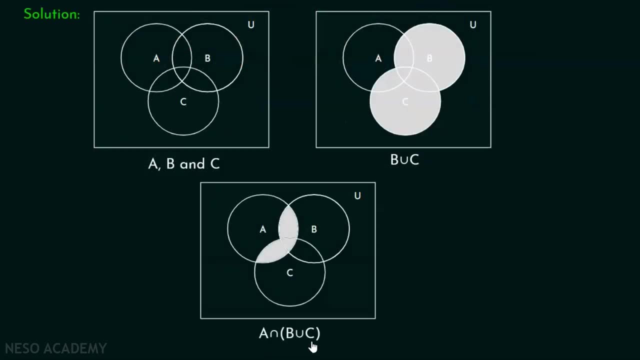 And B union C. This area, as well as this area, Right. So the Venn diagram for the same looks like this: This is the Venn diagram for A intersection, B union C. This area, as well as this area. This is the common area between A and B union C. 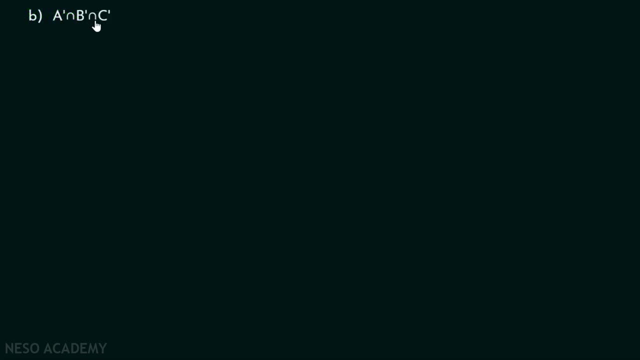 Right: A complement, intersection B complement, intersection C complement. We want to draw the Venn diagram for A complement, intersection B complement, intersection C complement. For this we will first draw the Venn diagram for A complement intersection B complement, intersection C complement. For this, we will first draw the Venn diagram for A complement intersection B complement, intersection C complement. 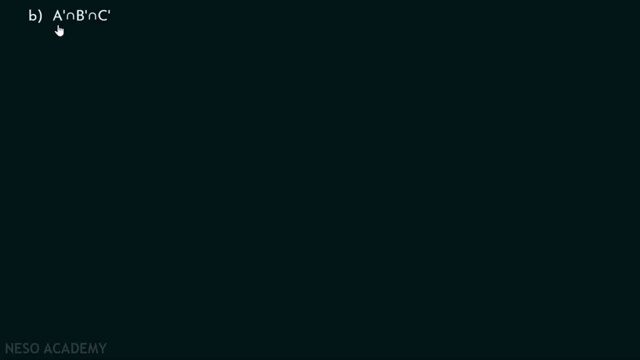 then B complement, then C complement, and then we will draw the Venn diagram for A complement, intersection B complement, intersection C complement. Let's just try to draw the Venn diagram for A complement and this is how it looks like, Right. 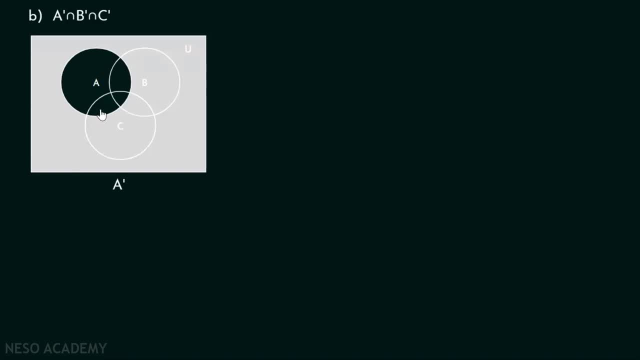 A complement means everything except A. A must not be shaded. Everything must be shaded, Right. This is how it looks like. What is B complement? Everything except B, Right. So every region must be shaded except B. This shaded region represents B complement, Right. 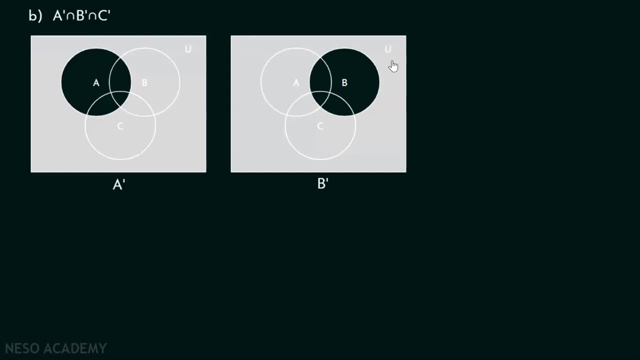 Even universe of discourse must also be included. What is C complement? C complement means everything except C. That means every region must be shaded except C Right. And what is A complement, intersection, B complement, intersection, C complement? We want to find the common area between: 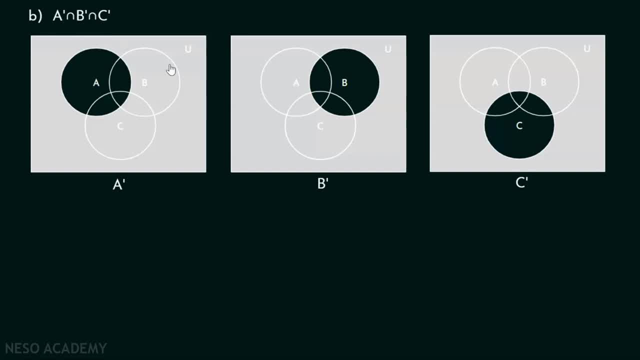 A complement, B complement and C complement. Now you can clearly see that this area is not common between all three of them. This area is also not common. This area is also not common between three of them. Obviously, this area, this area and this area. 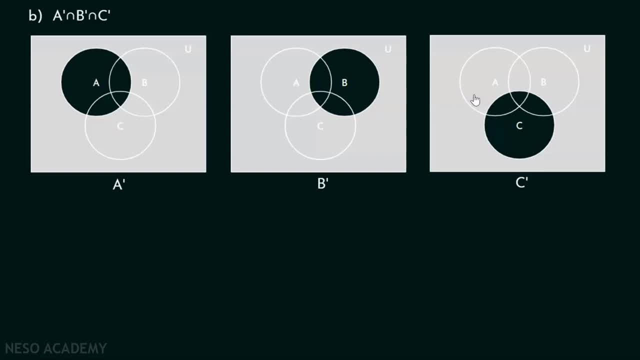 is also not common between all three of them. Right, There is only one area which is common between all three of them. You can see that this outside region is common between A complement, B complement and C complement Right. So A complement intersection, B complement. 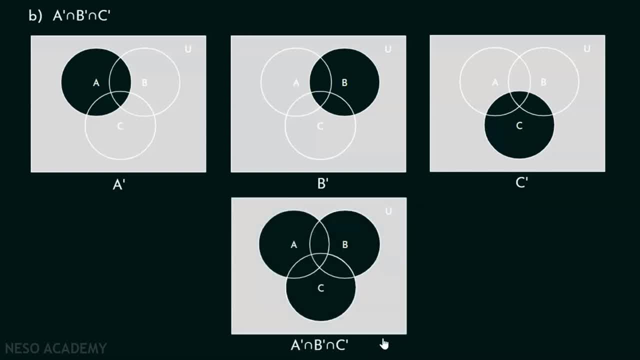 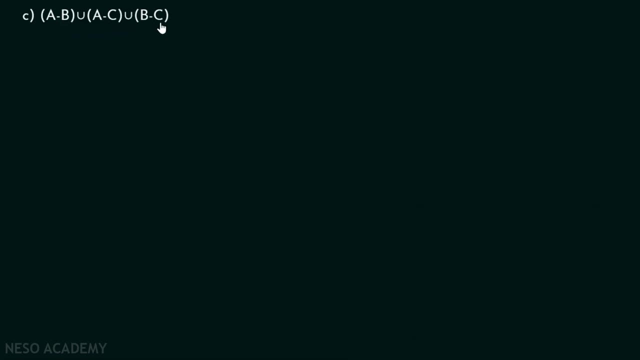 intersection C complement is represented by this Venn diagram. Here you can see this shaded region is A complement intersection B complement intersection C complement. Now how to draw the Venn diagram for A minus B union A minus C. union B minus C. 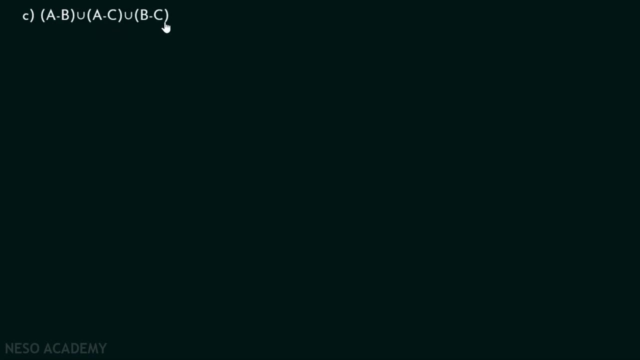 First we will try to draw the Venn diagram for A minus B, A minus C and B minus C. Then we will draw the Venn diagram for A minus B, union A minus C, union B minus C. Let's just try to draw the Venn diagram for A minus B.